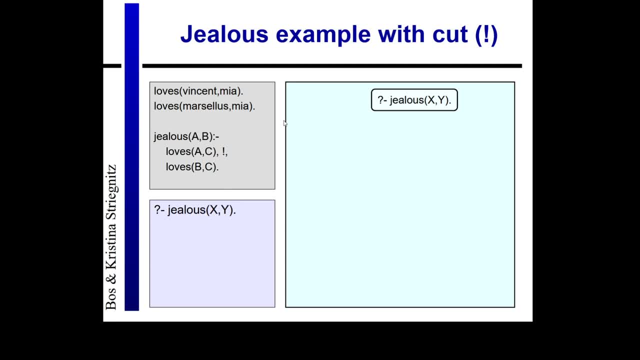 Vincent and Marcellus is jealous of himself. So we have four different results here And what we want to do is trim that list down. So the way we're going to write this is we have the old predicate we were working with- jealous AB, loves AC and loves BC- but we're going to put 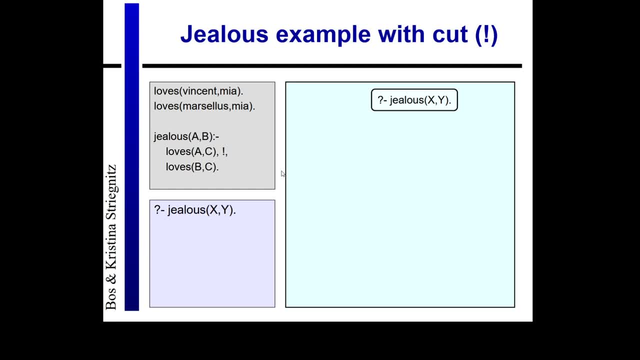 an exclamation point in between. So let's see what this results in. So we look at our decision tree. We try jealous XY. It matches with our predicate here: jealous. So X is unified with A, Y is unified with B. 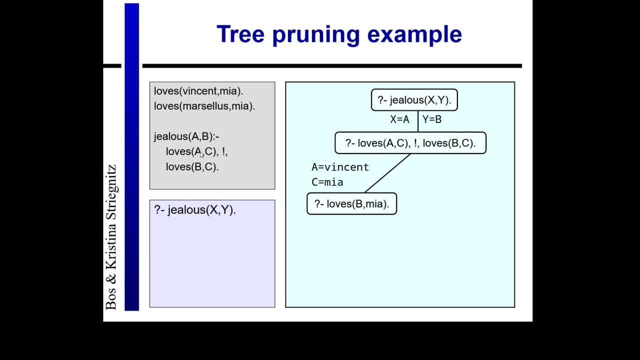 And then we go into our check: Is this possible? So loves AC. So the first thing we check is Vincent and Mia, And so if A loves C- this is potentially plausible with Vincent and Mia- Then we're going to pass our cut, which always succeeds. So we just go ahead and check. loves B and C? Well, C is Mia. 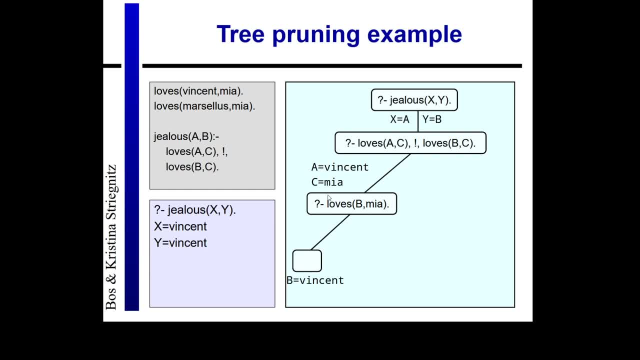 So we look for who else loves B, And in this case Vincent is our answer. So Vincent loves Mia, and Vincent loves Mia means that X and Y can both be Vincent, So he is jealous of himself. And while we're still down here on this part of the tree, we can check another B, C, Marcellus and Mia. 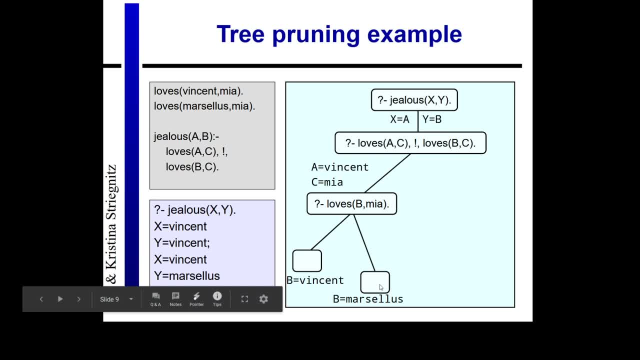 And so now Vincent is jealous of Marcellus, And this is the part where we would backtrack up. So we found all the combinations of A with A, Vincent and C, Mia. We found all the different combinations of B and C that work, And so normally what we do is backtrack, back up. 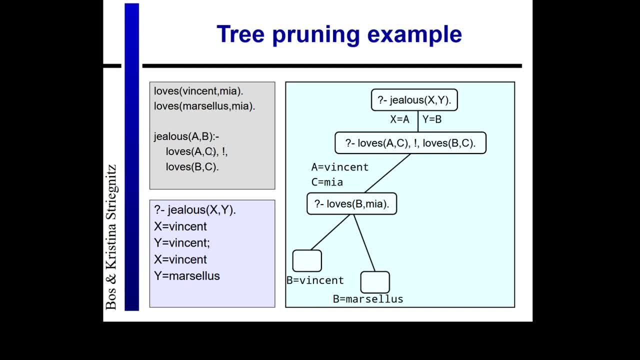 try a different A and C, in this case Marcellus and Mia- and then find out that Marcellus is jealous of Vincent and Marcellus is jealous of himself. But to get back up there we have to go back through this loop to go try a different A and C. We've already been down this path, So now we're. 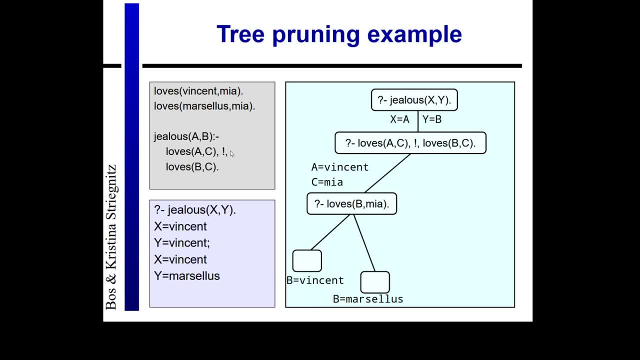 trying to go back up and go to the other path, But this exclamation point is like a little barrier there And so we can't backtrack. So that's the basic operation. Sorry about the extra flip there. That's the basic operation of backtracking. So this allows you to trim your tree and only have specific results.